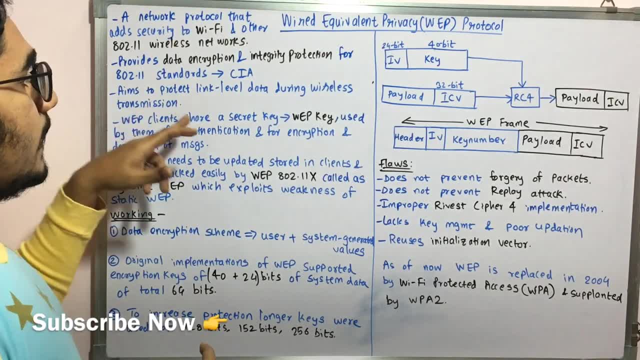 Next, this WEP protocol aims to protect the link level data during wireless transmission, means all the data which is being transported at the second time And image data which is being brought to the same set of keys are coming to the three-ижig free acabar 1 % data batch proxy with its data. 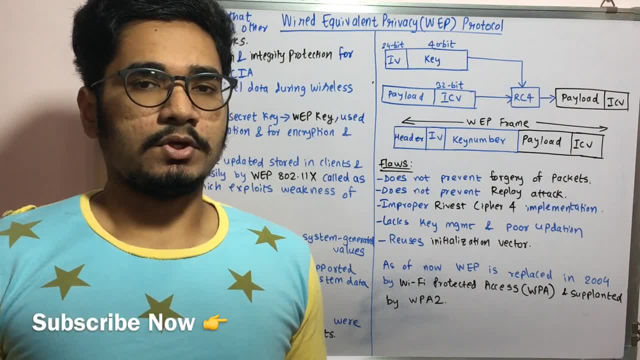 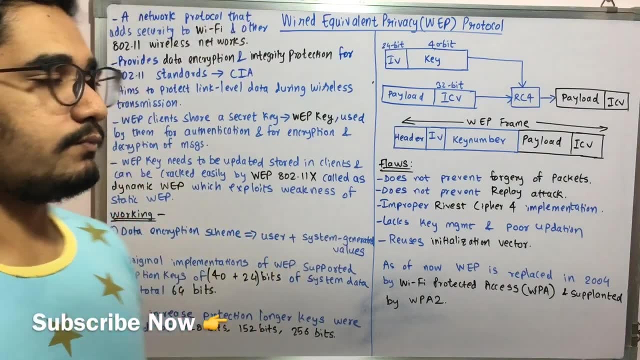 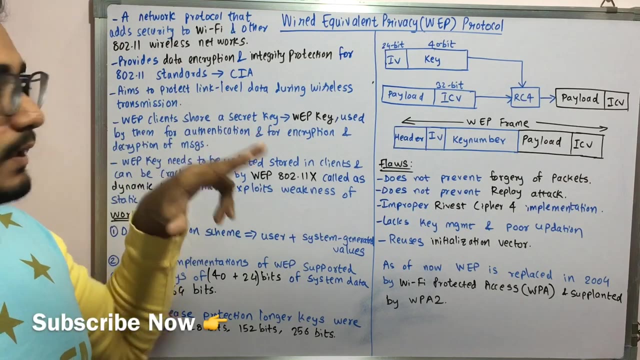 The WEP protocol has já set up a folder for the that as恐l Meir dot ph martyussy tape. this is the Kata data Linc layer, word by that phrase, structure from flim be guards being carried to individually frames ethically, they tell you. You know, should you keep the security. 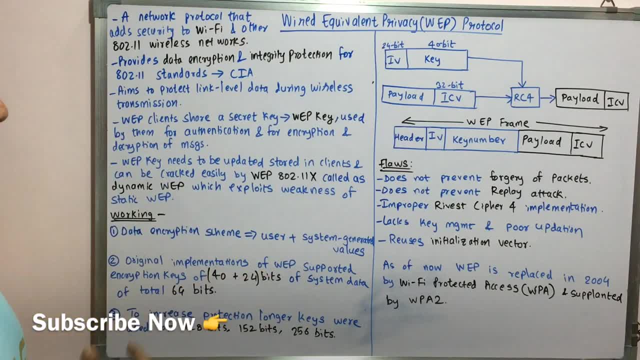 And so is this also a feature WP clients are. their great share is image data backup. teammates withinha have third key to keep a close top The secret key, so does not call US WEP keys. I have just got their collaborative Made this clothes. 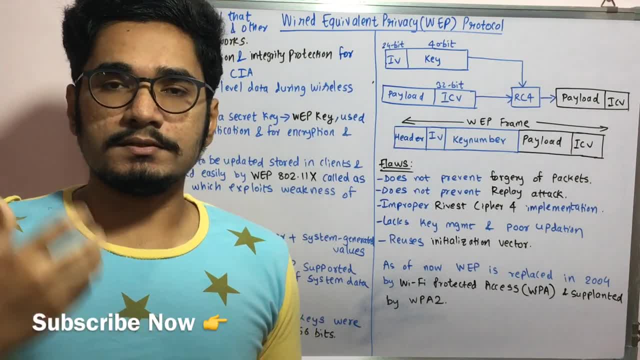 injection and also to work, and so lead bi Sherman virtual machine to bass. so this WP clients have got the set Also over a bending air when we're going to go through the things that are available- WEP keys- and so they share a same set of secret keys. and so next, if tomorrow, if any data transfer, 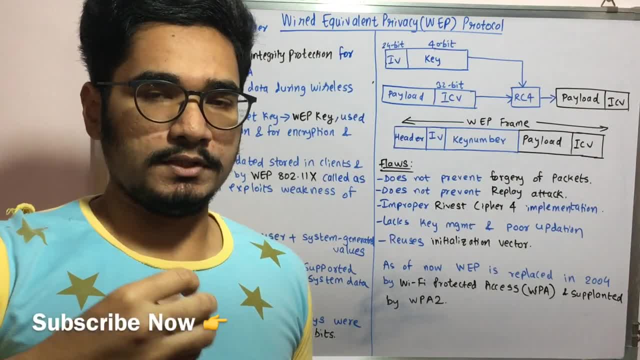 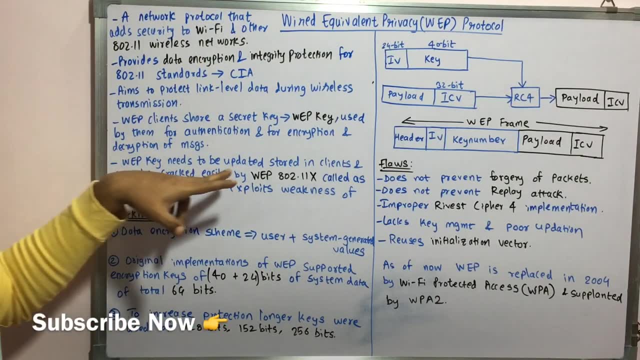 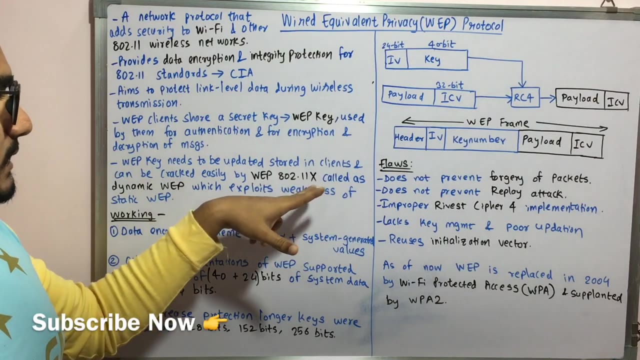 has to be done over this wireless network, then they use this kind of keys for encryption as well, as similar kind of fashion is used for decryption as well. So WEP key needs to be updated and it's stored in the client and can be cracked easily with the help of WEP 80.11x, which is called as a. 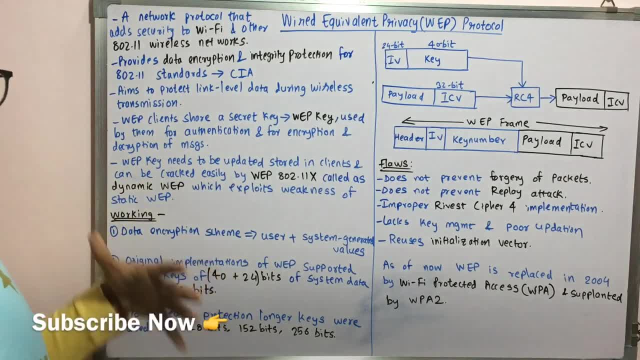 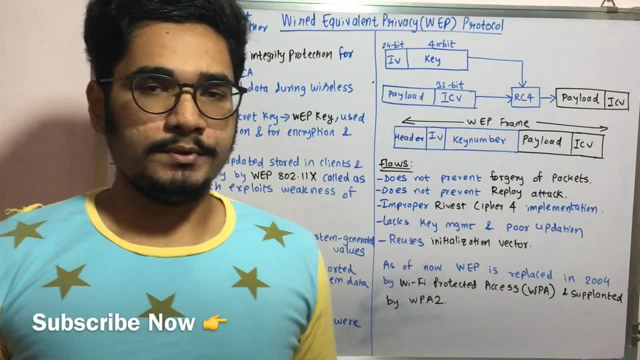 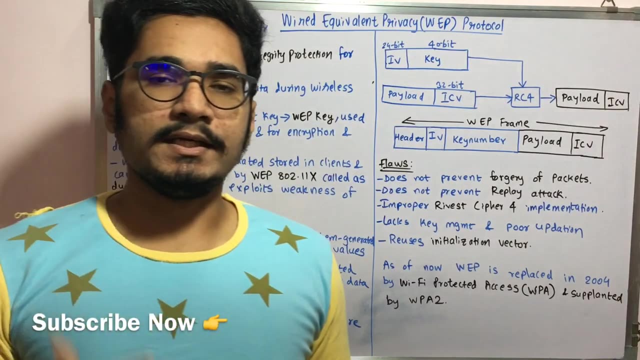 dynamic WEP, which exploits the weakness of the static WEP. So WEP itself has got two variations, that is, static WEP and dynamic WEP. So static, dynamic WEP has got its own limitations, where static WEP can be easily cracked with the help of dynamic WEP with 80.11x as its code name. 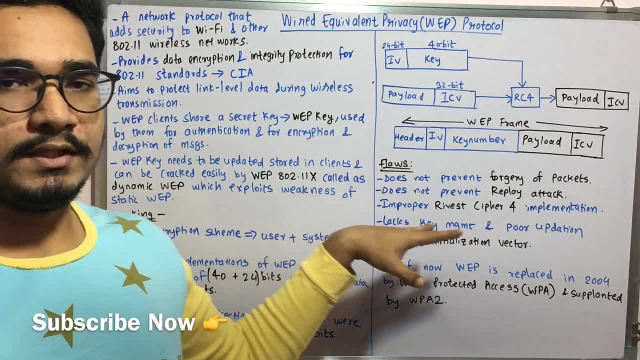 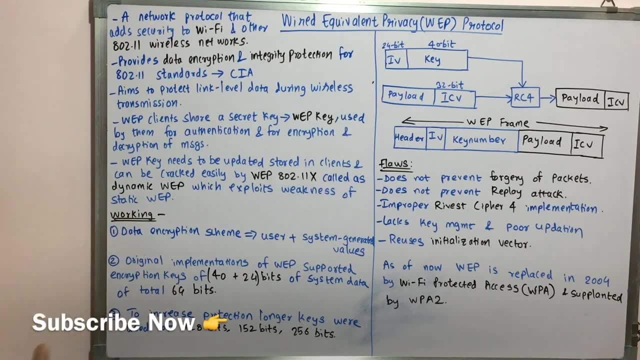 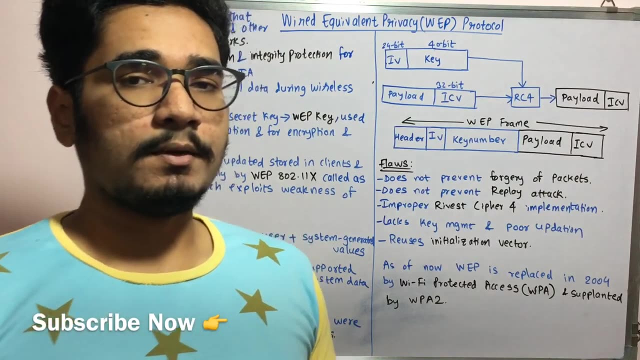 So it has got certain kind of weaknesses that we'll see. what are the various flaws which are there in WEP? So, basically, the working of WEP is in this way. So first, the data encryption scheme is there, So where you have the user generated values as well as system generated values, So those two values are being 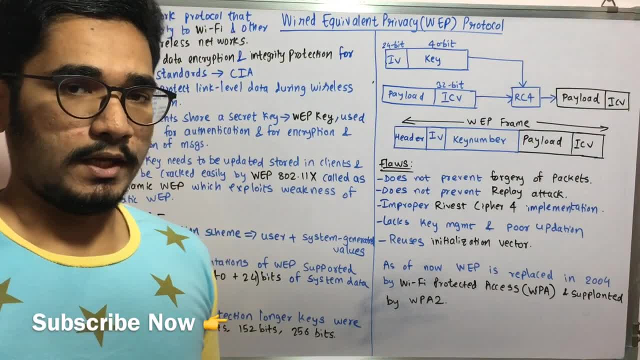 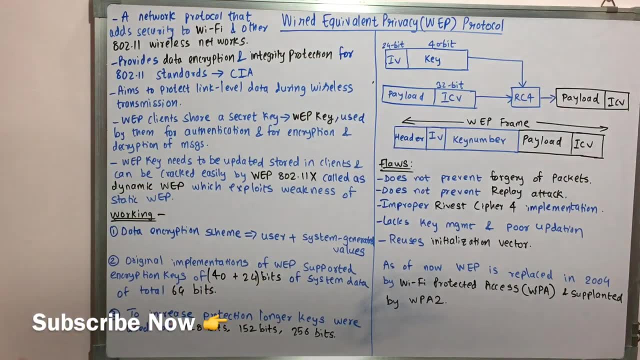 concatenated or which are being combined and then it's being applied to the algorithm. So a kind of RC4 system is there: Revest CIFR, and through that it's being generated. And so original implementation of WEP supported system. it supported encryption keys of 40 plus 24 bits. 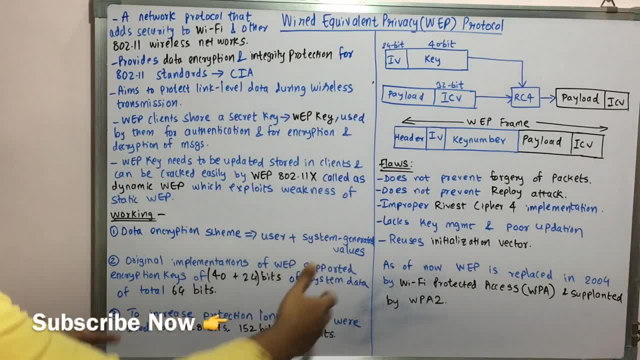 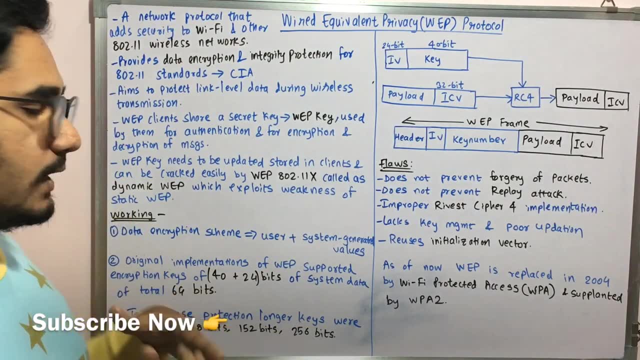 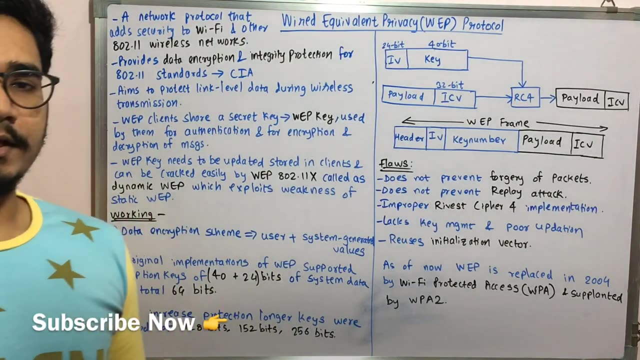 It's user and system generated bits and system data of about total 64 bits. So this makes a total of 64 bits. So originally this much was the data bits standard which were used. Now, tomorrow, they thought that if this gets confirmed or if any challenges appear, then they need to increase the protection level, and so longer keys are introduced of 128 bits, 152 bits and 256 bits. 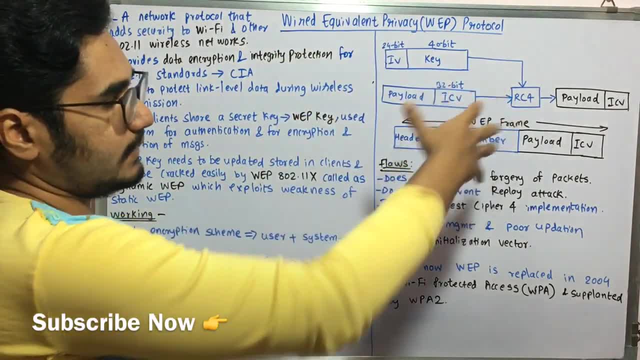 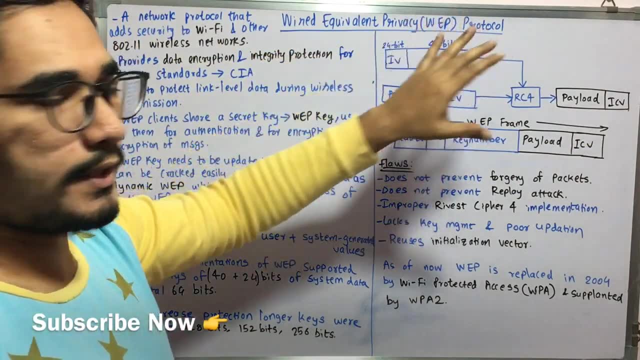 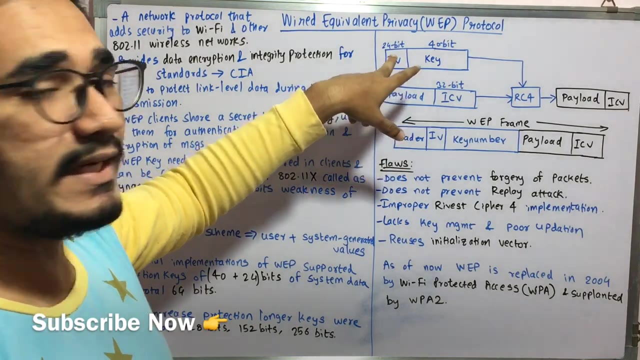 Now let's see the framework, Or how the data is being encrypted, or how the WEP frame looks like. So basically, to begin with, we have 24 bit and 40 bit, two different set of values or two different fields. So that is first. one is IV, that is Integrity value. 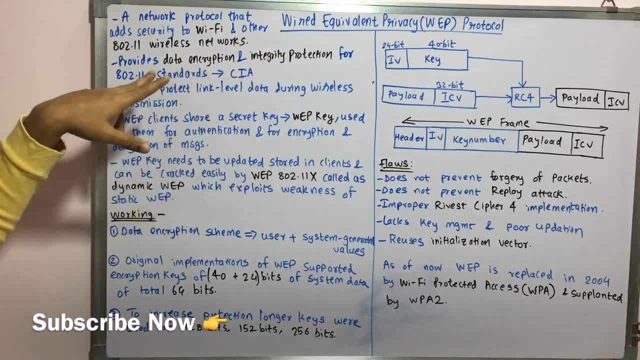 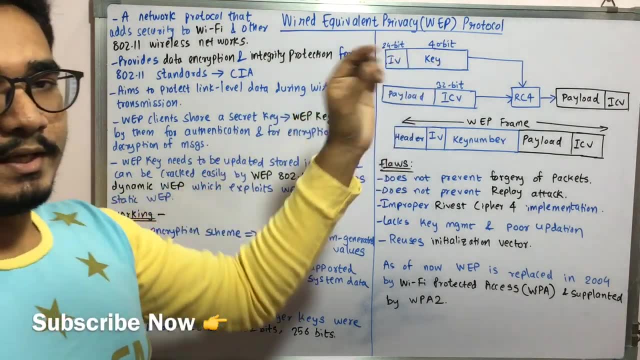 So in WEP we know it is used for Integrity protection and data encryption. So for Integrity protection we have this IV and then you have the key, which is this WEP key. So key has particular number or key value. So those two are just fed to this RC4.. 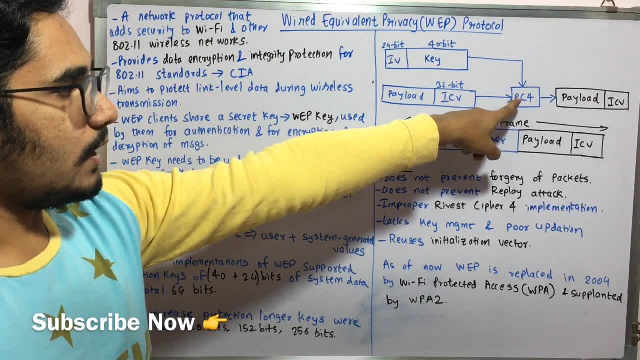 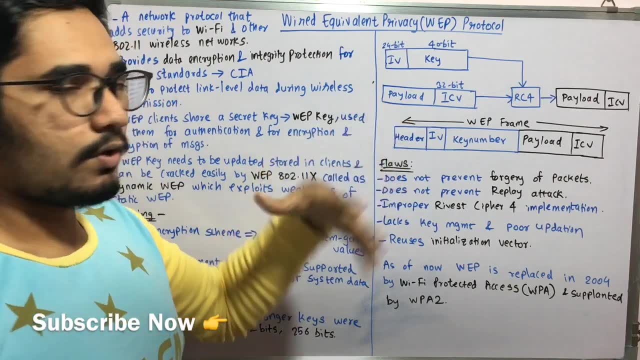 So this is a Revest Cipher, So this is an encryption, just combiner, and then you have this payload. Payload means the actual data which you need to send, whichever your data might be, whether it's a text data, or whether it's a visual or audio data. 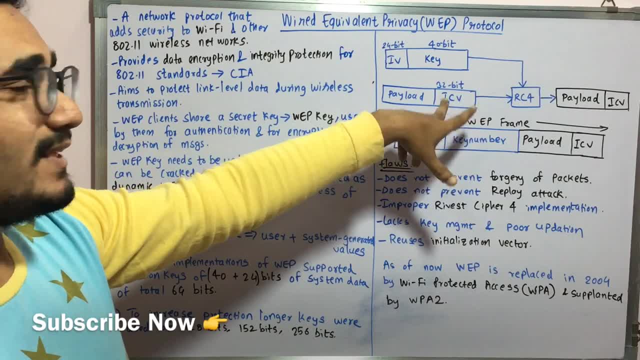 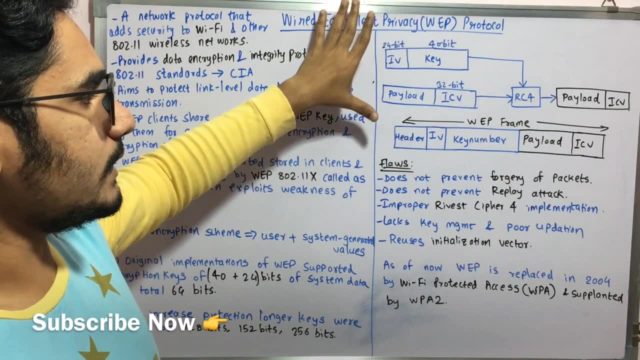 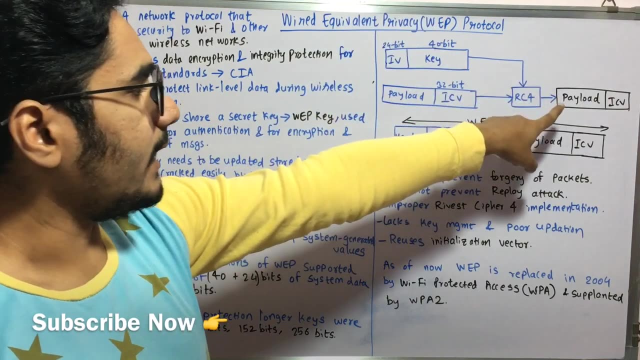 And then this ICV is used, that is of 32-bit. that is the Integrity check value ICV, which is now this part. all is unencrypted or de-encrypted. Then if you pass all these values to this RC4, then this part just get encrypted and it just forms a layer on this payload and ICV. 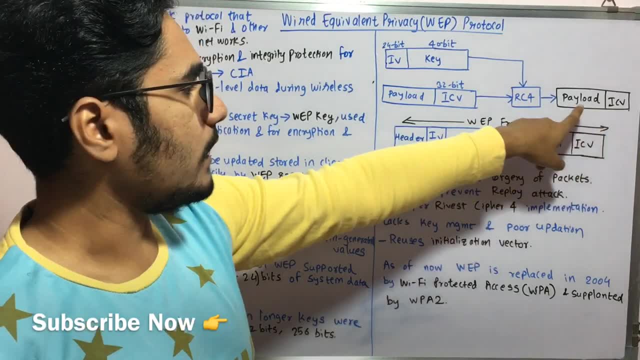 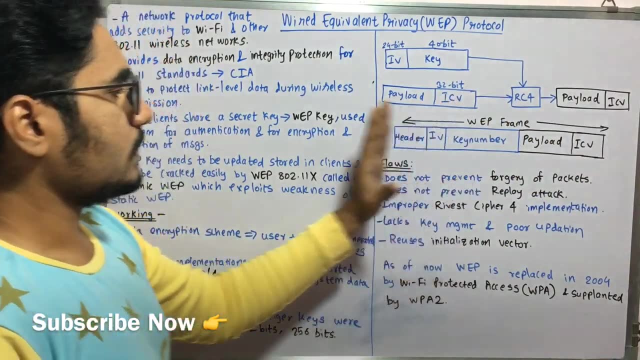 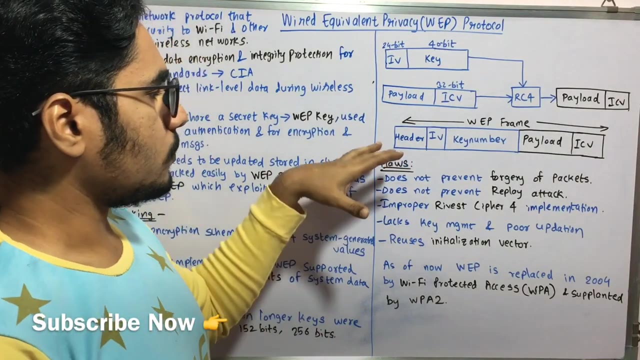 So at the output you have this payload and ICV value which is being encrypted. Now this encrypted value is attached to a set of three headers. So the very first one is the normal header where you can have the version number of the WEP frame and also other basic details regarding 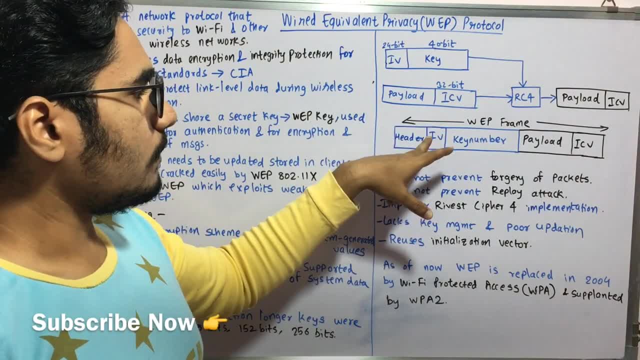 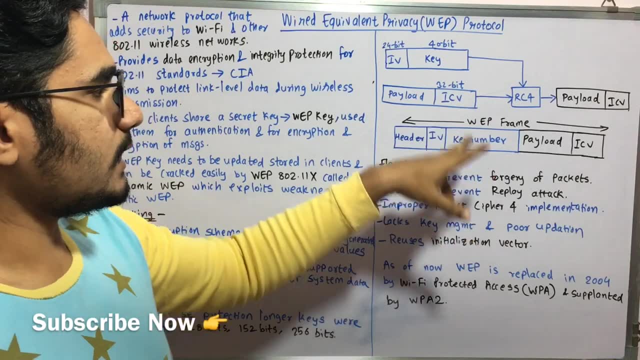 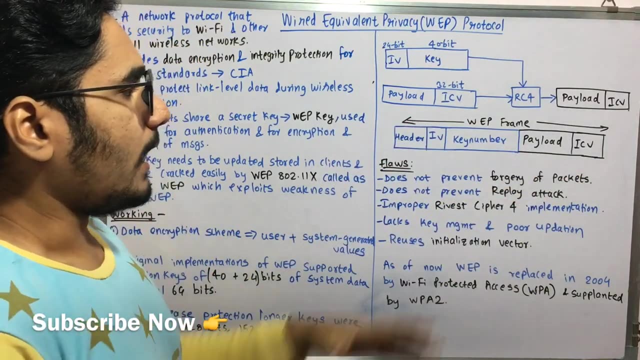 that WEP frame and next is the Integrity value, where you have the Integrity check being done and the number of times it is being versioned, and then you have the key number. key number is basically the key which is being used in series, So it's in a chronological order where you get the key numbers and then you have this payload as well as the ICV which you get from this step. 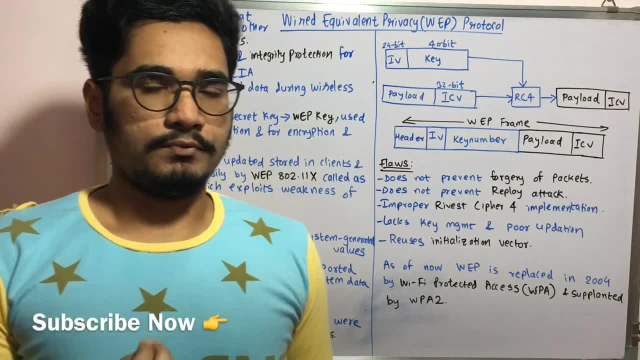 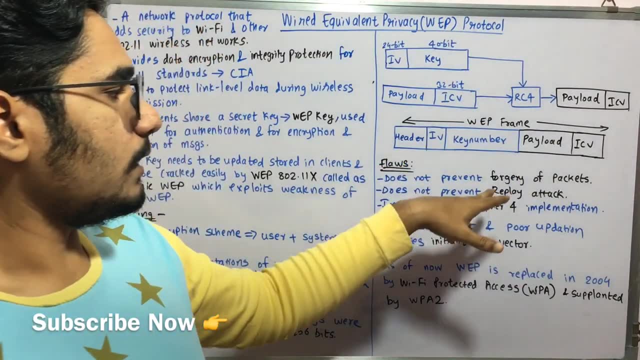 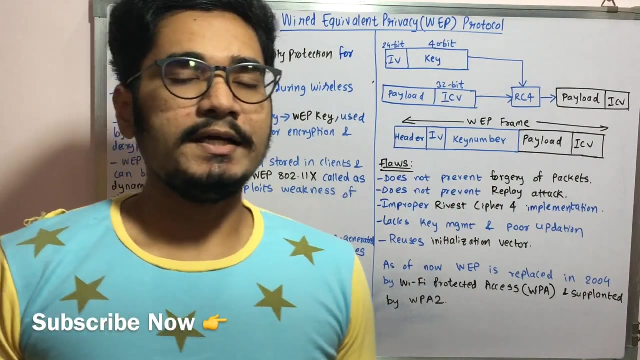 Now we told that in WEP there is a kind of flaw or it fails to check on certain parameters. So those are. it does not prevent forgery of packet, So mainly the network forgery happens. So forgery is nothing. but it basically does not checks any kind of validations over this packet. 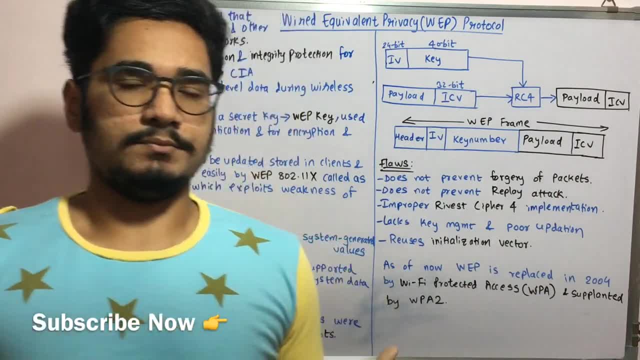 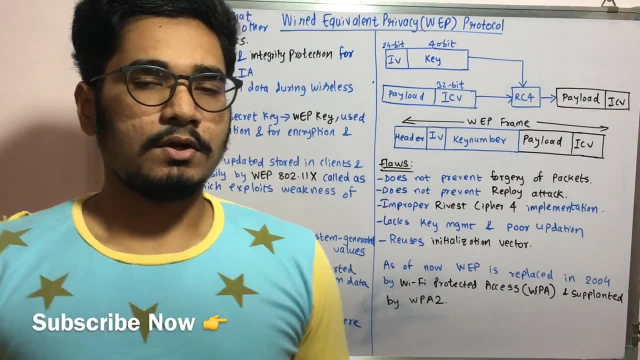 It just accepts the packet and sends to the end system. So at the other end, if there is an attacker being present and if it's being done with evil intention, then it's not possible to identify with the help of WEP and the sender who is sending this information will get compromised. 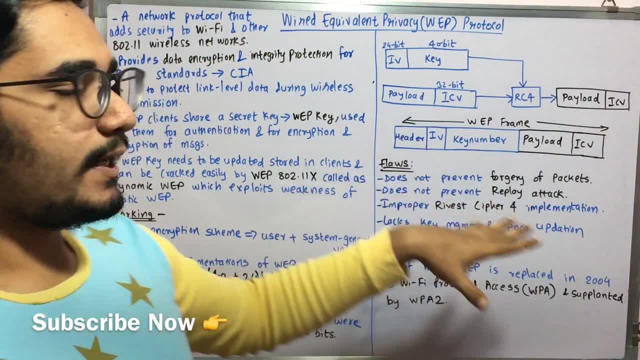 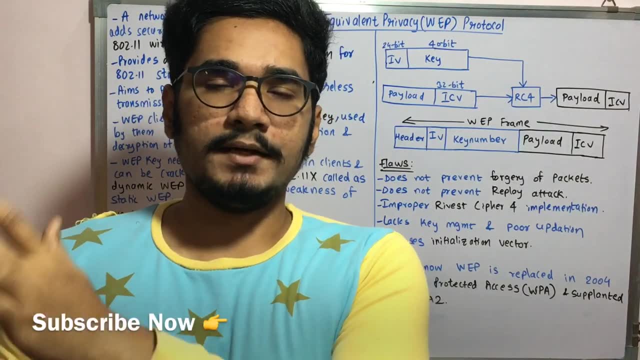 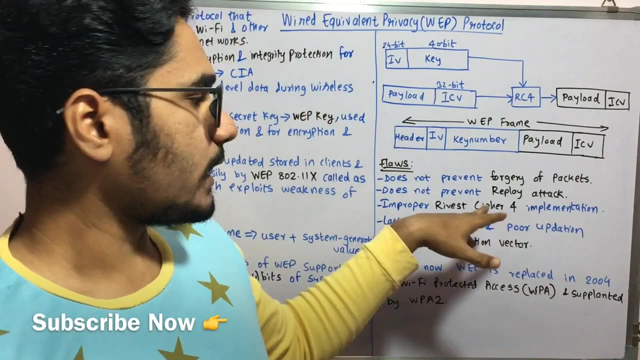 Next is does not prevent any replay attack. So replay attack is basically: first you record a particular scenario, Then that scenario is being just replayed back and the other system will be under the impression that it's been coming from a valid, legitimate system. So those kind of checks are not done in this. 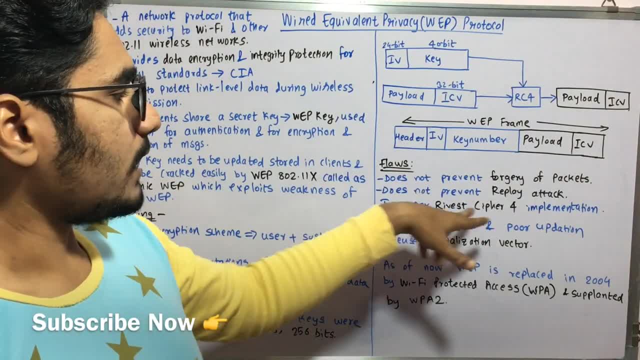 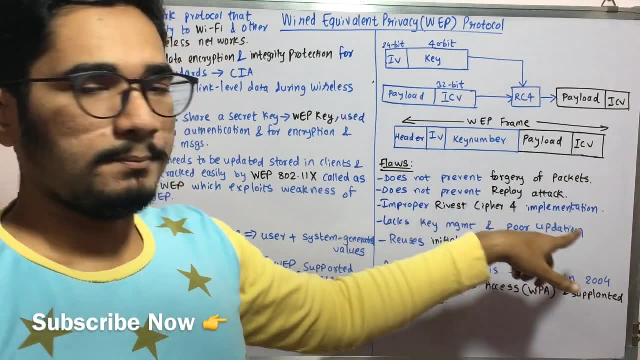 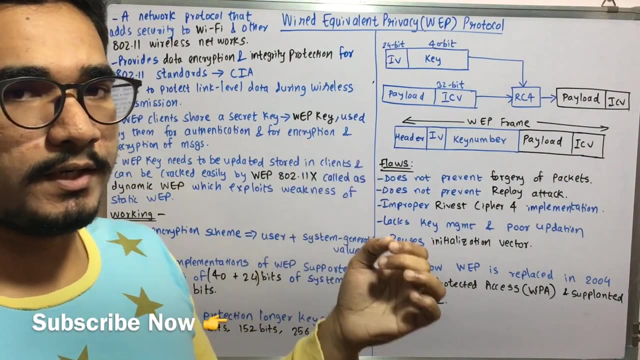 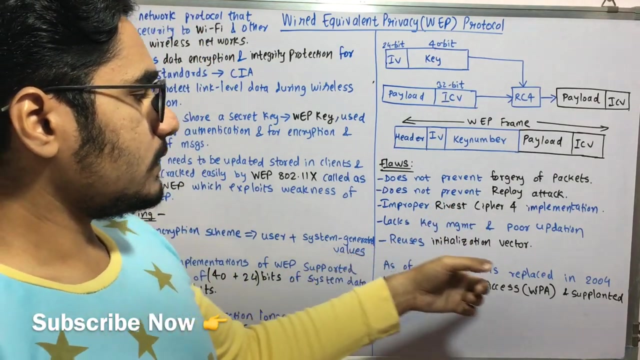 So it's prone to replay attack and there is a RC4 which is being used here. So this RC4 used in this is very vulnerable And so it's done Under improper implementation. So that kind of issues also there in WEP. and it lacks key management, since all the keys are shared among different WEP clients and there is no proper or the updation is very poor in this, and so it reuses the initialization vector. 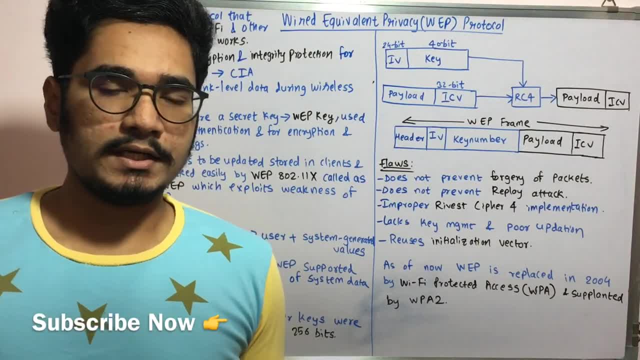 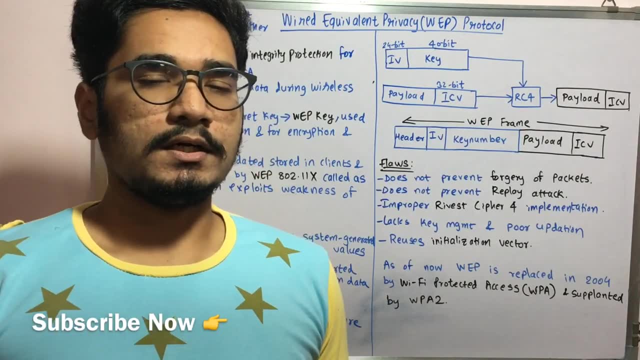 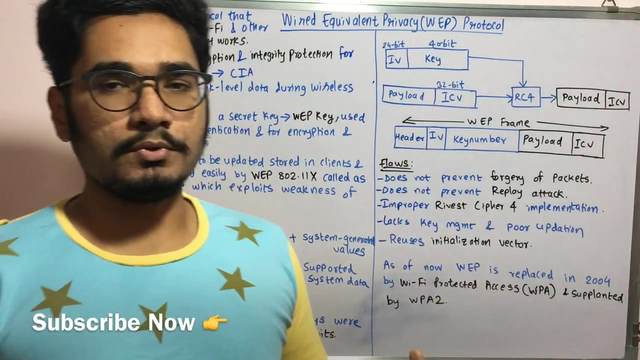 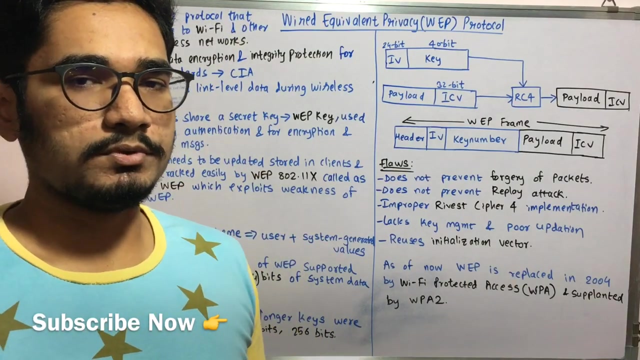 So initialization vector is basically when we generate a particular WEP frame, you have that matrix or that vector, So that vector it does not basically checks for any other hardcore Decryption technique. So you can also use the brute force attacks and any free internet widely available software can be used in order to decrypt those kind of data. 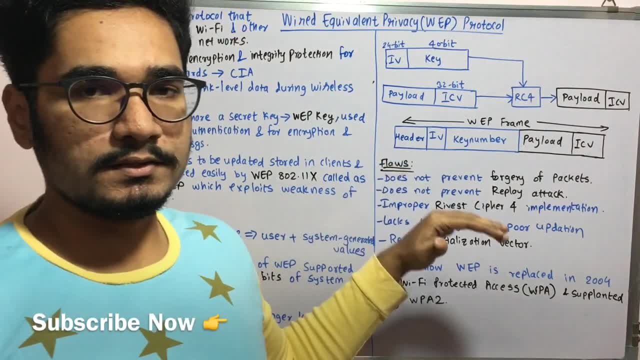 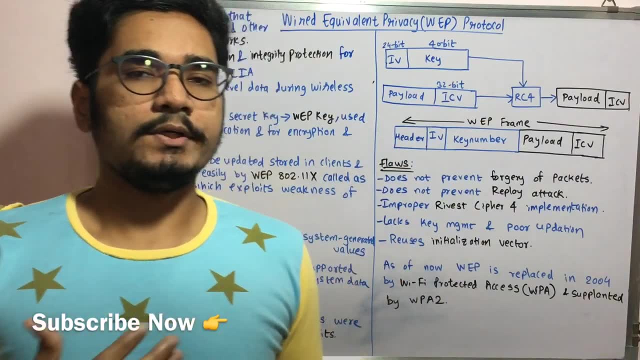 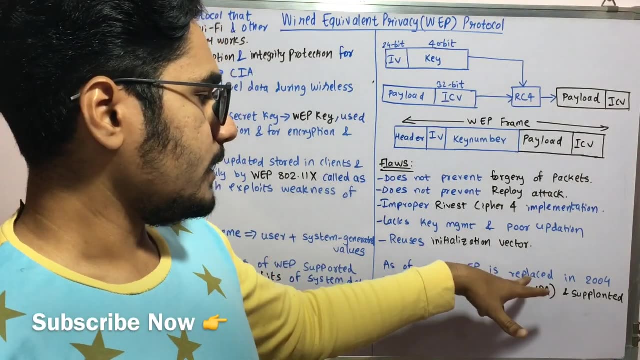 So it's not that very secure. And so, if this kind of protocol is this much vulnerable to attacks and it has got so many flaws, you need to formulate or you need to come with another protocol which is used for Wi-Fi systems, And so, as of now, WP is not there and it's replaced. 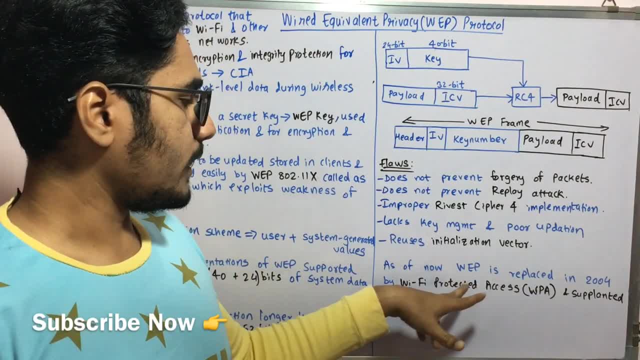 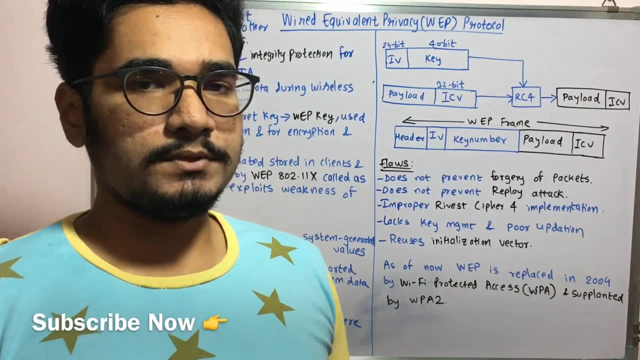 In the year 2004, with the help of Wi-Fi protected access, which is called as WPA, and it's supplanted by the WPA 2 now, in all of this Wi-Fi systems, You will get this kind of WPA. So I have got an example.